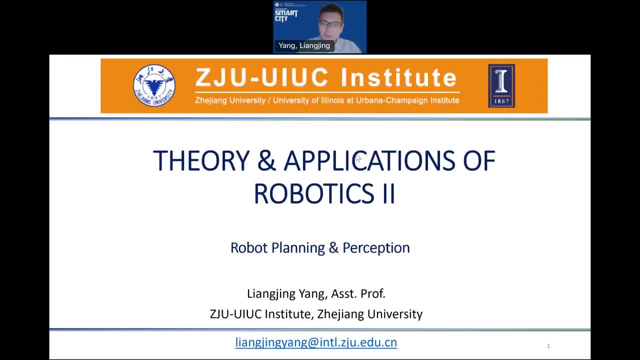 All right, welcome back to theory and application of robotics tool. All right, so if you're seeing this video again, I'm probably still in the hospital, right, Uh, but uh, That's uh, go into some of the more applied topic about uh, robotics. 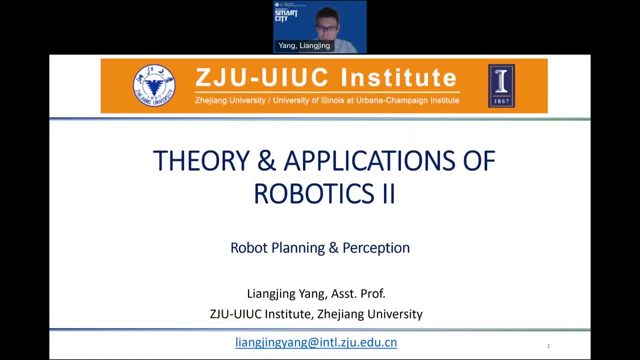 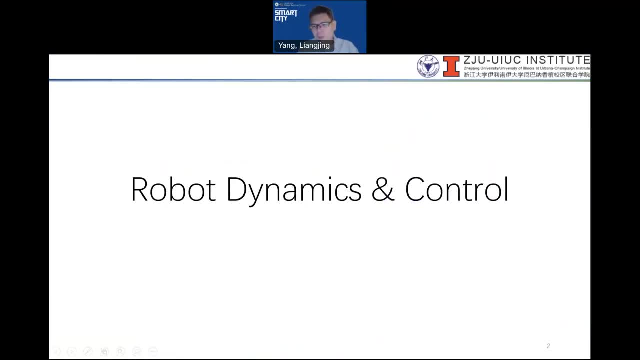 Okay, something that we can look forward to, okay. So now that we have actually covered all the Uh essential fundamentals from dynamics and control, Okay, We are able to relate it better in actual robot application. So when we put a scope, 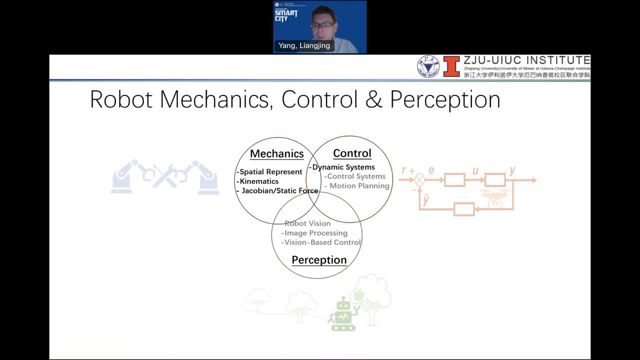 Around. we see that, uh, combining mechanics, control, and later on we're going to see perception To close out the loop so that I can interact with that problem. So previously, uh, in fundamentals, where you look at the mechanics, you are understanding the plan itself. 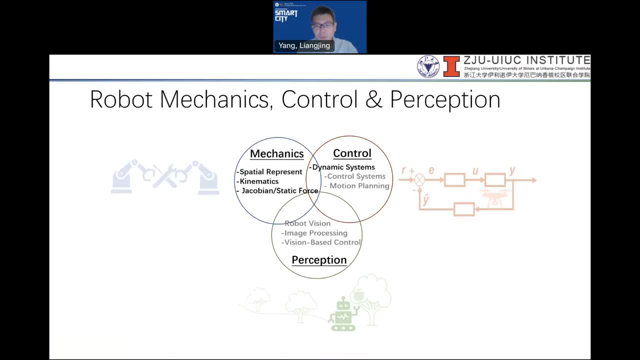 How do you actually model the plan? So, uh, being able to represent it mathematically, So that you can analyze and come out with solution. and then, uh, in our 1st uh, or rather 2 days back. 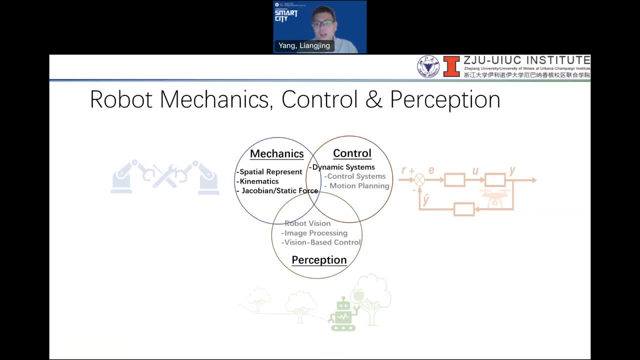 Uh, we actually look at control system. how do we actually uh achieve the target that we want? So remember, robot is uh nothing by machine designed to achieve certain tasks while interacting with the environment. So you kind of need to understand uh the task as well and how you go about achieving it. 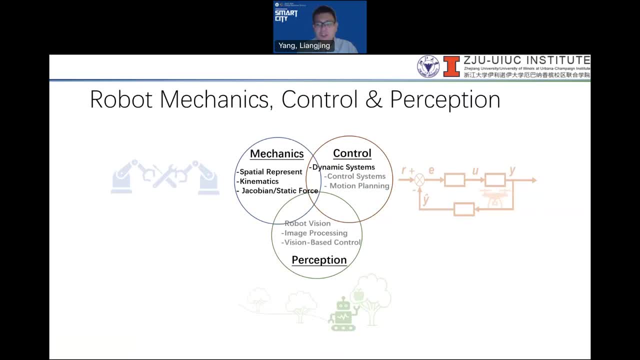 While interacting with the environment, so you need perception, Okay, So this is what we're going to Look at in this lecture as well. Okay, So, being able to uh understand, uh, images Of the surrounding allow the robot to able to react. 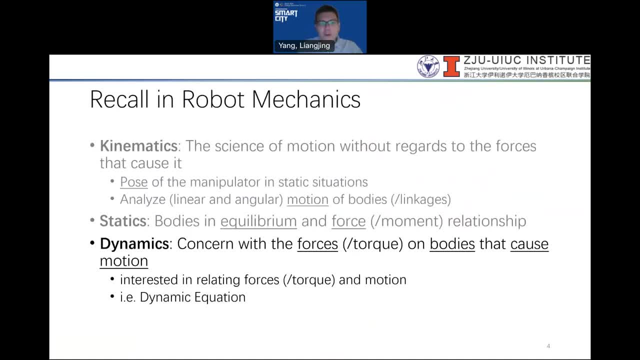 To the environment. so let's recall our robot kinematics. Uh, we actually went through kinematics, static body and dynamics. We're going to have a very quick uh Uh run through of it, Okay, Of course. uh, it doesn't do justice for me to just spend a few minutes on this topic. 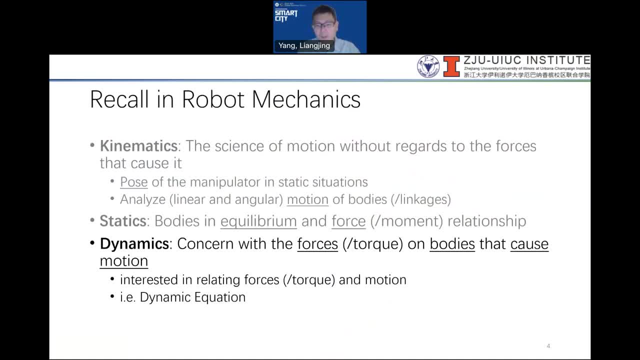 Okay, but I'm just going to uh relate to what are the relevant uh Aspect to the context of robotics. Okay, so in this case, we are interested in relating the force and motion. So what are the forces that causes this? Oh, that caused this motion. 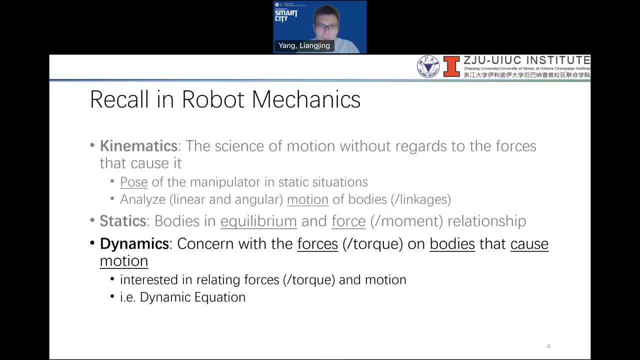 All right, so we need to work out the dynamic equation, All right, Uh so, uh, there are some example to keep you motivated. Okay, When you design a robot like this. uh, computer robot. Okay, The MIT, She thought. 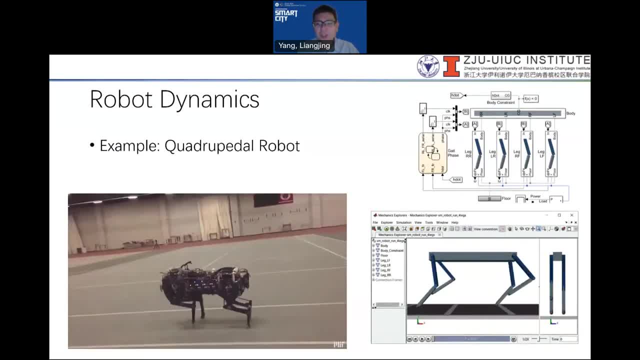 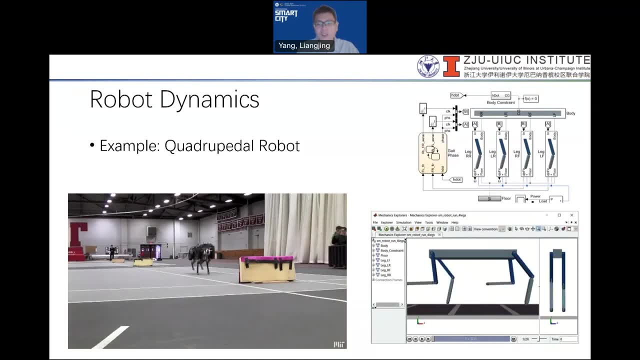 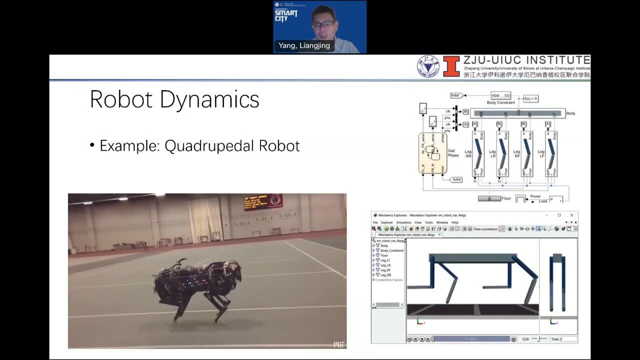 Okay, it's actually involving a lot of interaction with the environment, and some of these dynamics, Uh dynamics of the system, is actually very complicated, Okay, so, uh, modeling itself may not actually be Uh totally uh effective. we also need to have uh robust control. 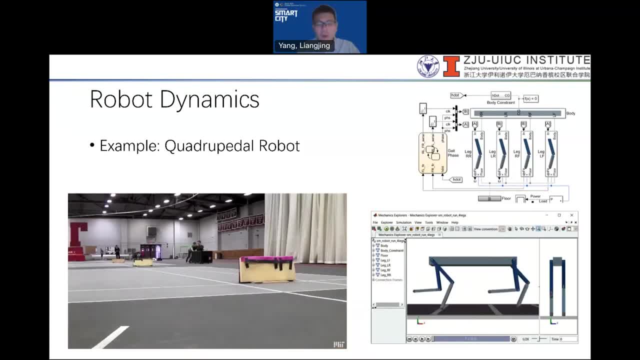 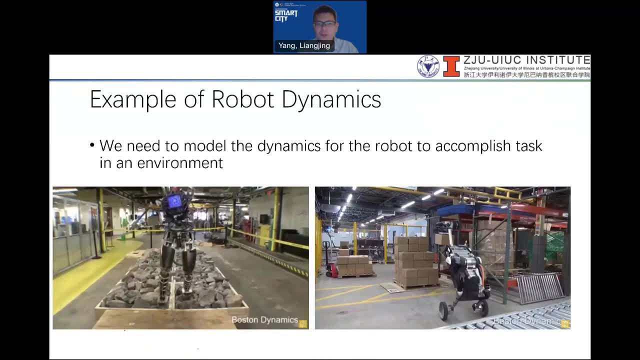 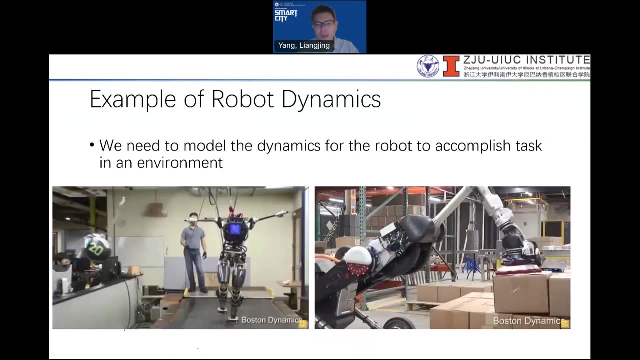 Uh, adaptive control to be able to make sure that robot is doing the right task, Uh, to achieve the right goal or the right outcome, right. So these are some of the example. I'm sure you have seen This. uh, for Boston dynamic, it actually went. uh, oh, it came a long way. Okay, Starting from uh, very prototypical, uh robot that couldn't 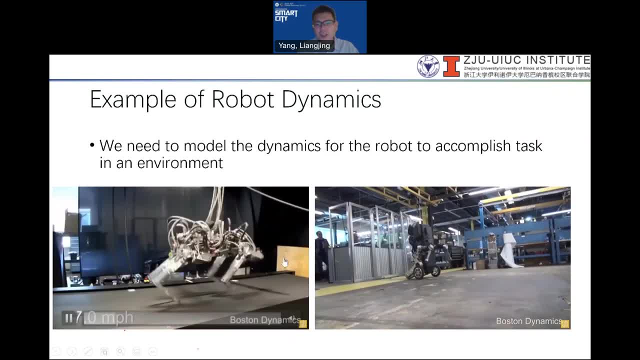 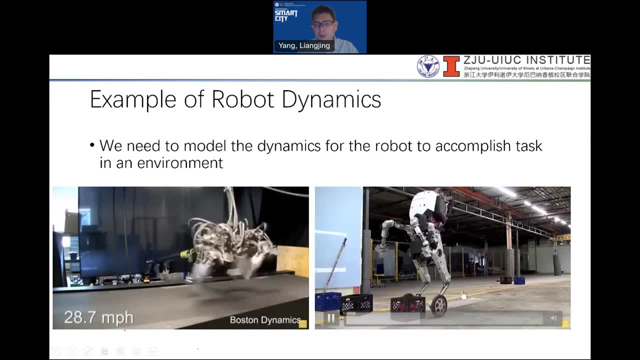 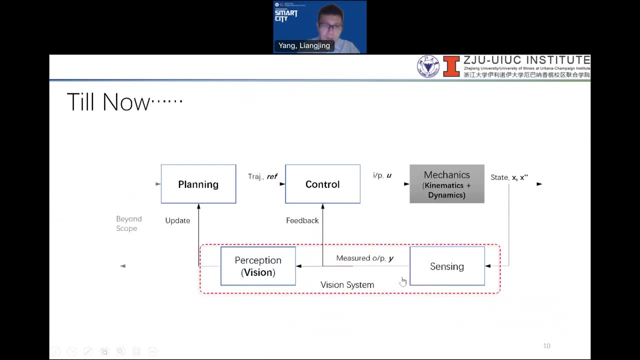 Uh, even perform very simple task, Okay, but today the robot can actually do superhuman task. Okay, flipping, and this is actually uh out doing a lot of, uh, human Expert, okay, the acrobatic capability, Right, so you know uh. 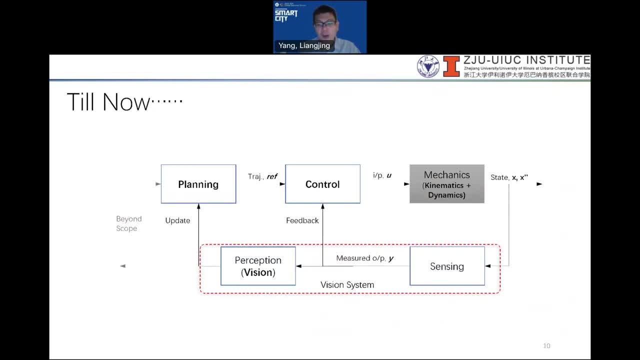 we have already covered mechanics, so we are able to uh, model or represent the mechanics. Okay, Essentially the plan When we talk about it in a control contact and we actually Roughly know what kind of control scheme that we can design to achieve the 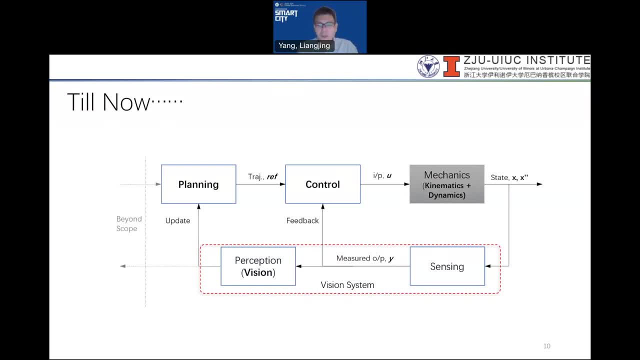 Uh, outcome that we want, Okay. So the next thing, of course, if we move up the level of intelligence? Okay, we actually wanted to be able to perceive the environment. So sensing, Or rather perception, is actually a higher Level of sensing. so when you sense, you get information. 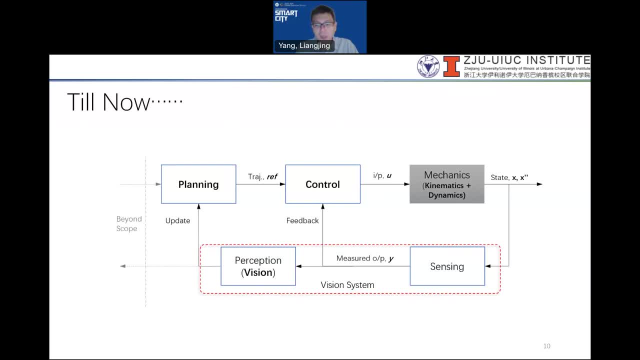 But you're not necessarily, you don't necessarily get Uh convert them into high level information that can do decision making. Okay, so that comes uh with Perception, and perception is actually something that will update your planning, So the robot can actually uh work out, plan Okay. 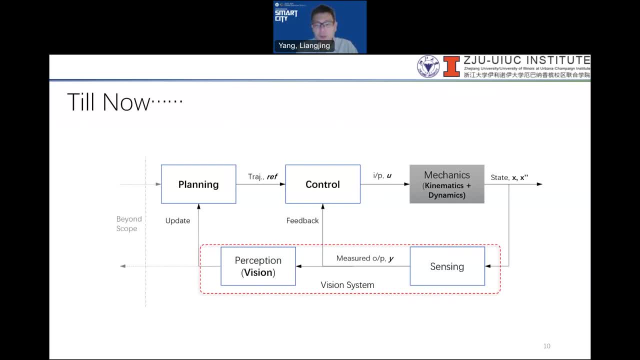 That uh will reach certain goal. Okay, so these are like trajectory: references come out with a trajectory, So how do you achieve certain goal? Uh, with a certain plan, and then you have this traditional reference sent into your controller. 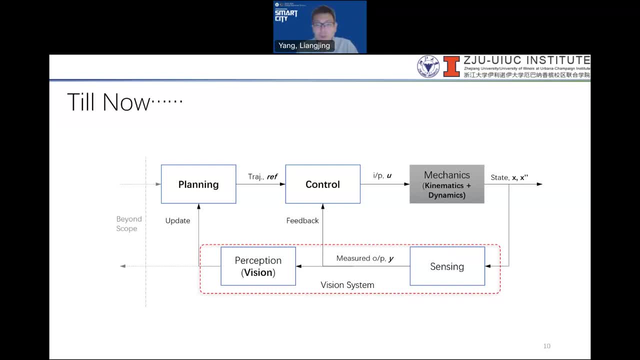 So that the controller know what kind of input You to send into your plan. Okay, There's a mechanics of our robot And then uh, through this uh interaction with the kinematics and dynamics. Okay, it will uh result in certain state. 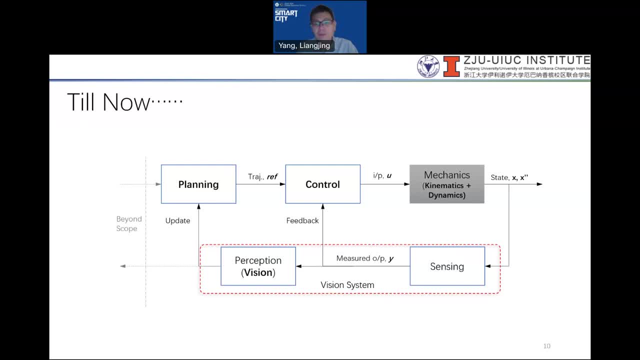 Okay, So that state could be sense or perceive and feedback into the control and planning. Uh, all right, so of course, anything beyond there, of course, more sophisticated, Uh, level of connection when you do decision making reasoning. 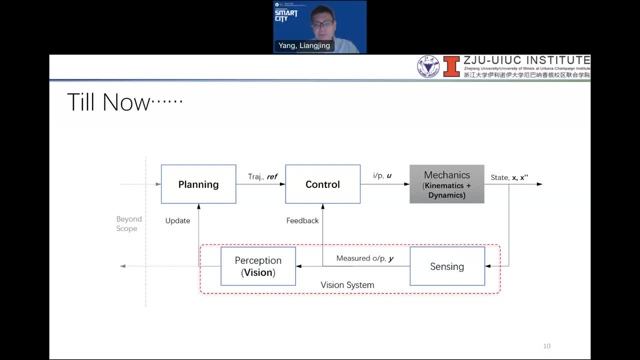 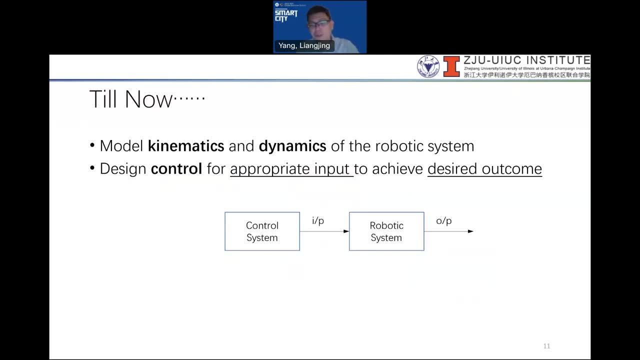 And that is actually not within the scope of this uh lecture. All right, so this is what I've been mentioning: Control system. tell you the kind of input that you need to send into the robot. Okay, Your robot is something that you already model. 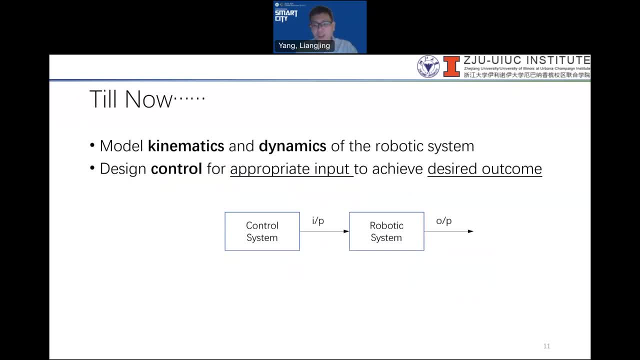 Remember your kinematics analysis. you are able to represent this robot And then dynamic, able to use a dynamic equation to uh Describe the robotic system, and then the control can actually come out of the input that will reach the desired outcome. Okay, so we're going to look at uh joint control. 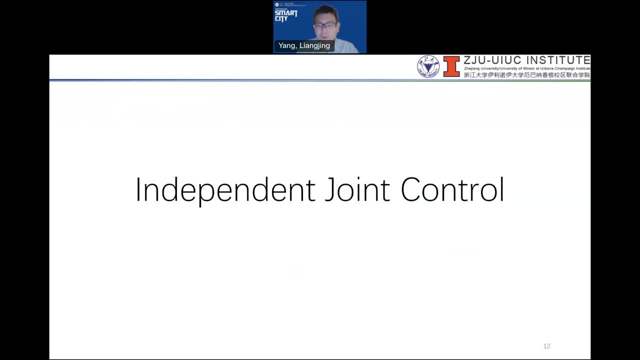 So, assuming that, uh, each of this, we are controlling the robot by? Uh using a model attached to 1 of the joint, Okay, So I will. Uh using a model attached to 1 of the joint, Okay, So I will. 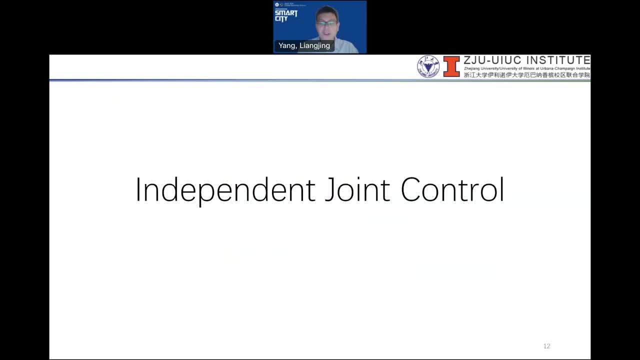 Control problem now simplified to controlling this joint. Okay, so remember earlier on, when we do for kinematics, uh, we have, Uh, we are representing the uh. This uh link: I with respect to Uh, I minus 1, using the transformation metric: I minus 1.. 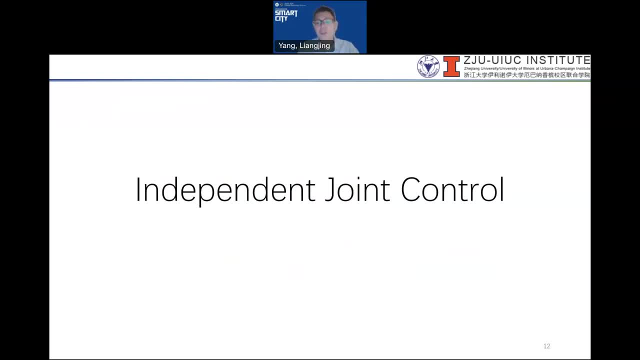 Okay. so uh, with that, uh, you kind of want to Have some form of input that you can change this Uh post right, So you need uh joint control, Okay. So of course in real life you can expand it to uh multiple. 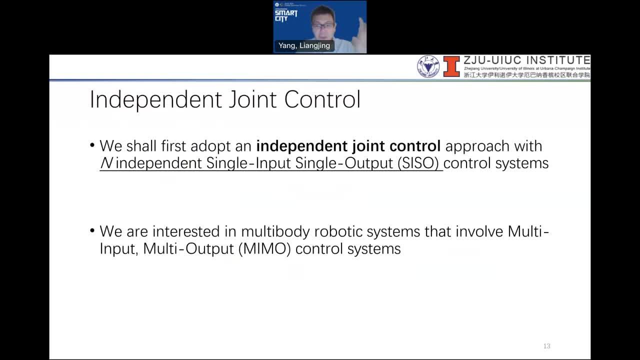 Uh, joints. okay, not just a single joint, but we start off with Creating a control scheme for only a single joint. All right, so eventually we might be interested in what we call, uh, my most system. Okay, Multi input, multi output control system. 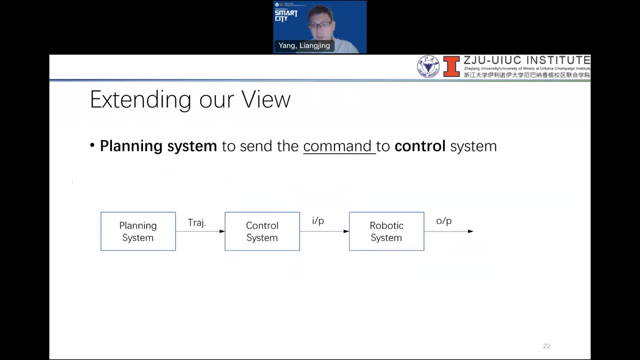 But in this case we're going to simplify The uh control problem into a single independent joint control. Okay, So the planning system. okay is when we are sending in the command Uh to the control system. so, strictly speaking, planning is. 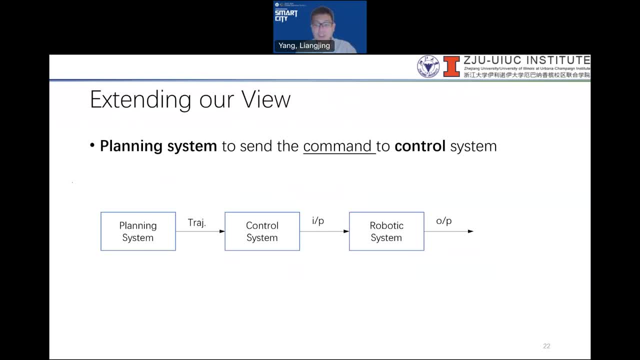 To achieve certain, go to the step that you would take, or designing the procedure that, Uh, you will go about achieving certain goal, So you will have certain goal. Okay, so you come out with a trajectory, so you want to move, uh, something from point to point B, while 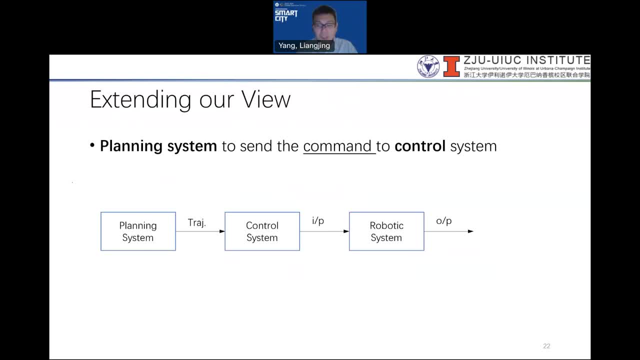 Uh avoiding certain obstacles. so you need a trajectory, Okay, and that is going to be sent to Your control system so that a controller will know what kind of input Uh for the actuator to affect your robot Uh, robotic system, so that you will uh achieve the desire state. 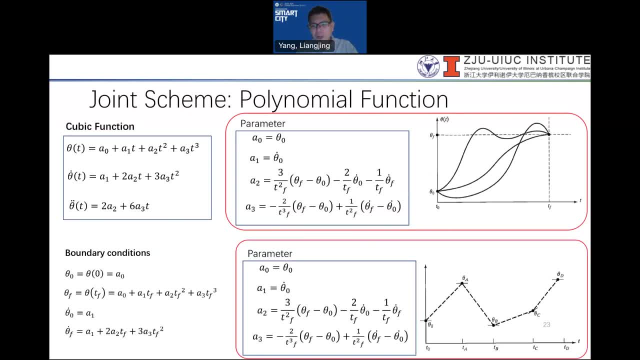 Okay, so there are a lot of methods here. Okay, I will encourage you to Uh look at uh John scraps uh textbook On some of these. uh function in trajectory generation Uh, but uh, due to time constraint and for a practical reason, 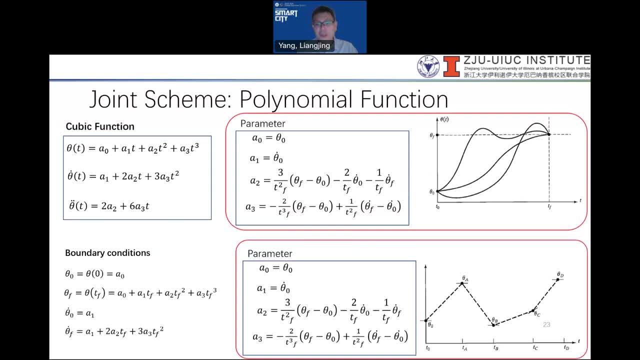 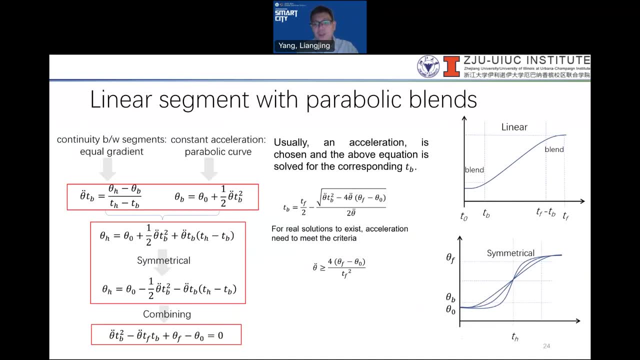 Uh, we are not going to go into detail for all these various function. Okay so, but uh, they are actually quite standard once you uh know how Uh different ways of uh generating your trajectory. Uh, it is not uh too difficult. 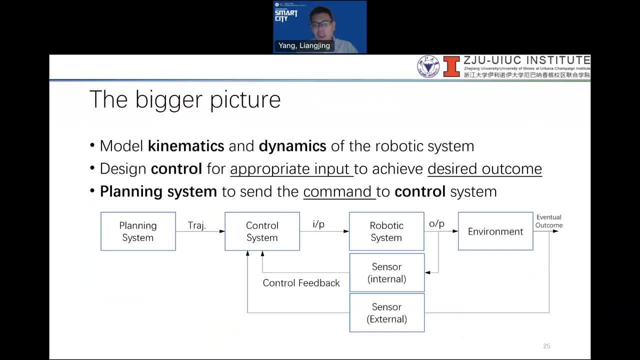 Okay, so the bigger picture, uh, that we want to, the bigger picture that we want to really look at, Is how, uh, we can combine all this to create this, uh, the design is Robotic system that help us uh achieve certain eventual outcome. 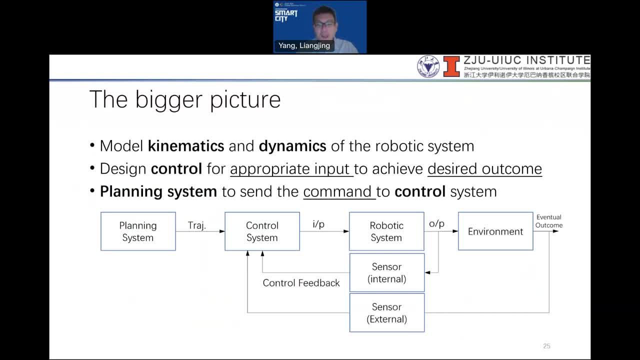 Okay, so you will have all these, uh, various component, Okay, planning control robotic system itself and the environment that it is working with. Okay, so, uh, of course, sensors are important Sensors and actuator, which we didn't cover too much here. 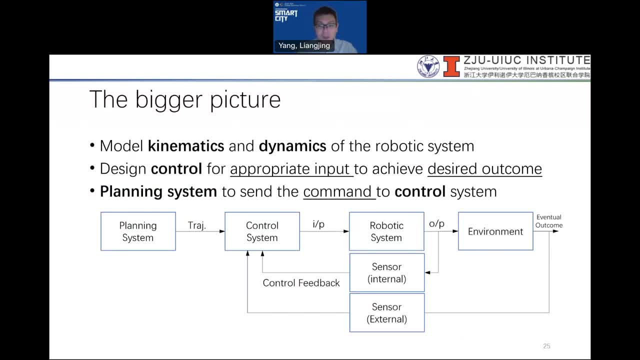 Okay, depending on your interest, you can actually go in depth, Uh, in looking at this uh branch of uh engineering called mechatronics. All right, So, uh, let's go on to uh robot planning 1st. 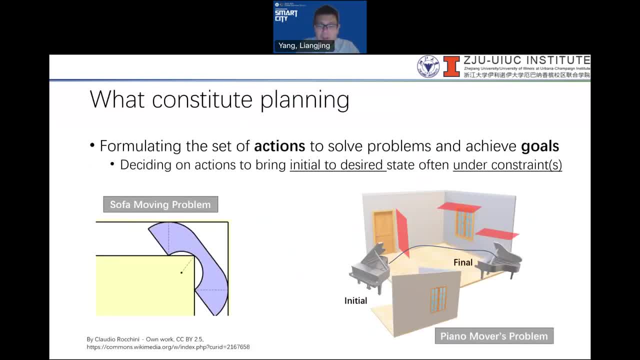 So, like what I mentioned, uh is nothing but formulate Uh or other planning. if you want to formally define it, it is formulating a set of actions that we need to solve a certain problem and to achieve certain goals. 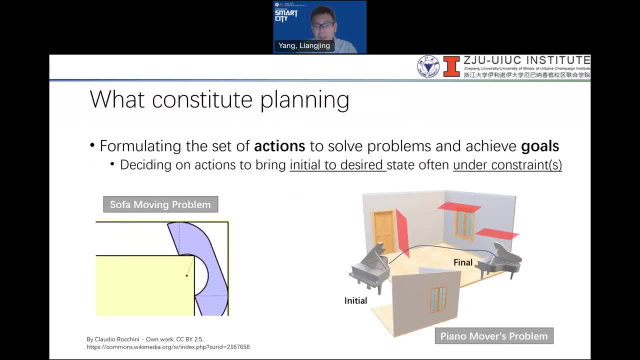 All right. so deciding on an action to bring Uh particular initial state to a A particular desire state, Okay, But often you are based with country- So it's not so easy- where you can do it in any Uh random manner. sometimes you are faced with country like this. so far moving problem. 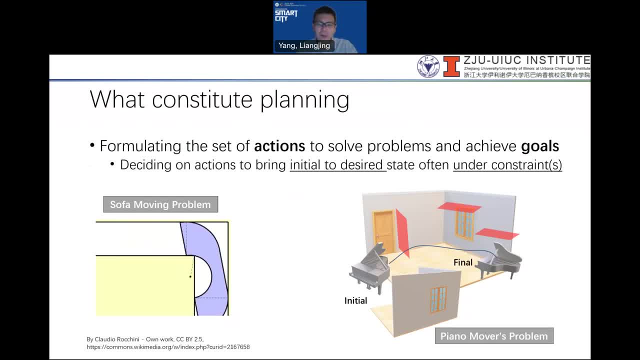 Okay, the piano problem. all these are uh very common or popular mathematical Uh problem. yeah, we have All right, you have uh initial and final position and you need to Uh then some of the obstacles. okay, avoid obstacles. 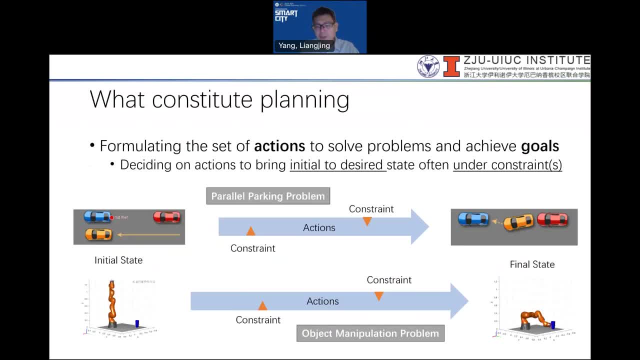 So parallel parking? Uh, it's part of the planning. Okay, You can't just shift, Translate your car directly into the parking slot. Okay, You need to maneuver it in such a way that, uh, it fit in, uh, parallel. 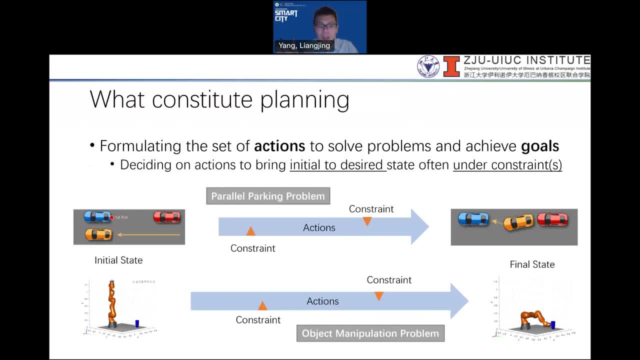 Uh, into the parking lot. Okay, So this is Coming out with certain action, Okay, While having the constraint. okay, so the same thing for robot. you're Uh going to do that sometime when you want to bring cup. 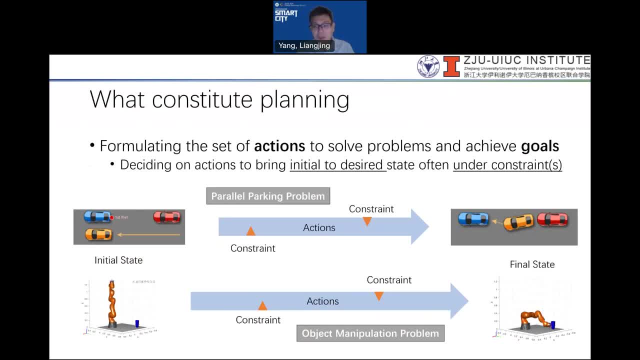 Say, for example, an object from 8.8 to point B. Okay, By the same time, there are so many way of doing that You want to optimize it, or you want to avoid certain Uh obstacles, uh, you are under certain constraint. 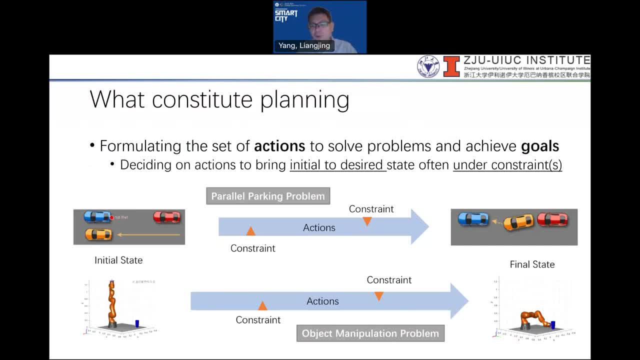 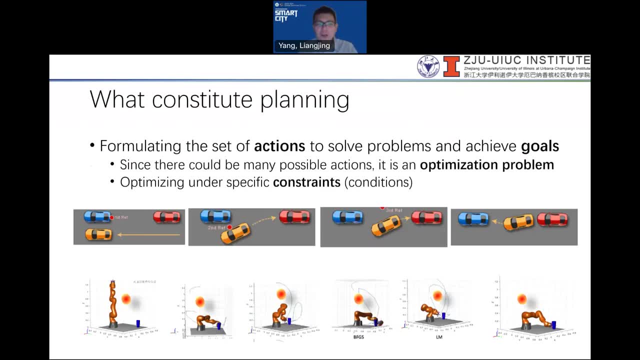 Okay, reducing the amount of energy required for each joint. Okay, So there are many different objective function. Okay, so these are some of the illustration. Okay, What constitute planning, formulating a set of action to solve the problem and achieve? 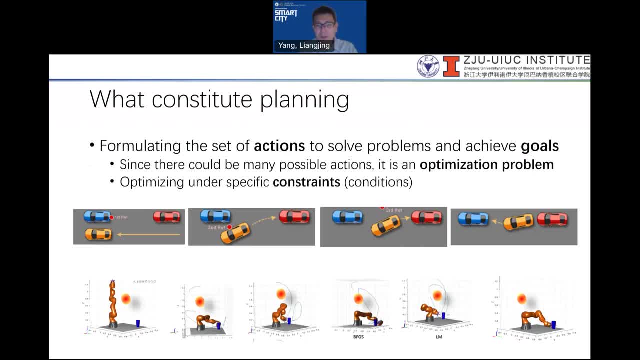 Goals, okay, since there could be many possible Actions. so this is actually an optimization problem, As we all know. so optimizing under specific constraint, All right. so we see this, uh, in a lot of example. Okay, Formulating a set of action, I want to 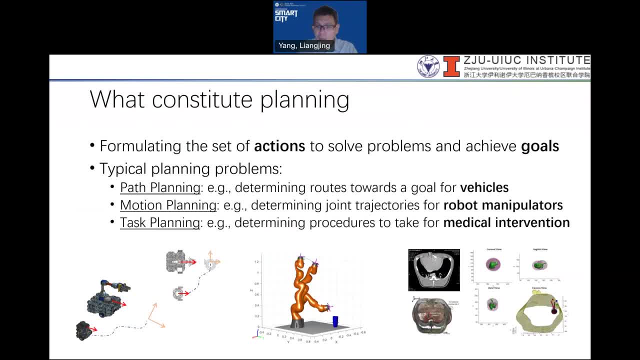 Mention. you want to solve the problem and achieve goal. typical problem will involve our planning. Okay, Uh, very common in robotics: motion planning, task planning. Okay, So you want to determine the routes towards a goal for, Or you want to determine a joint trajectory for, the robot manipulator. 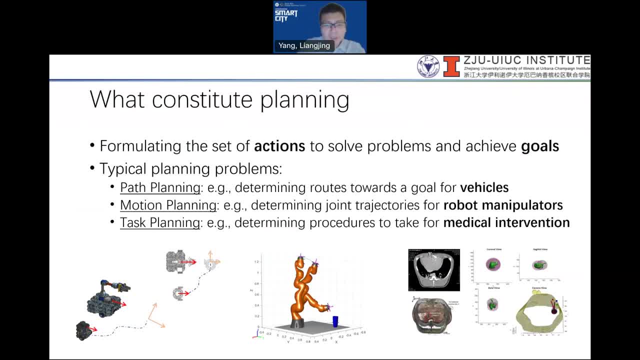 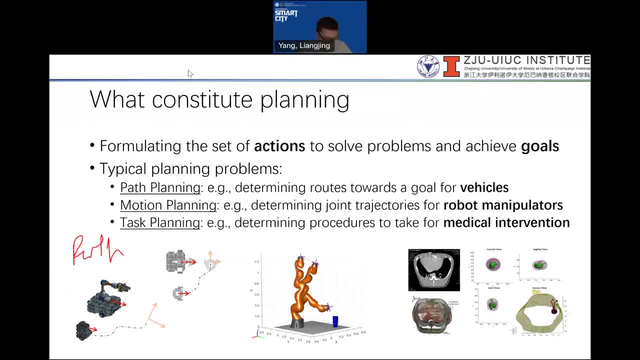 Ask me to get ready the ambulance coming. Can I continue to wrap up this thing? Okay, I quickly. Okay, so this is pop planning. Okay, This is actually your motion planning, right? Let me just very quickly and notate this motion planning. 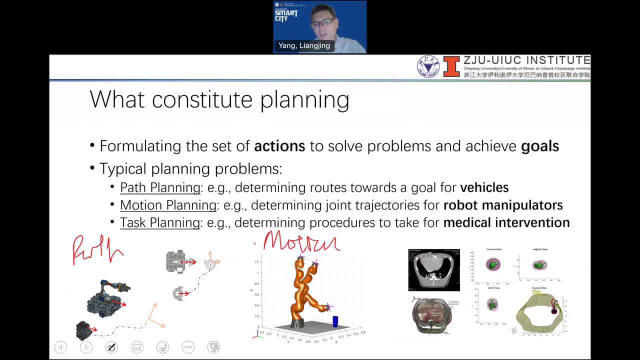 Okay, and at the same time, sometimes you want to define the task To do, especially the pace of medical intervention. I want you to see here: Okay, so this is cost planning. Okay, so there are various forms of planning. Okay, So sometimes we 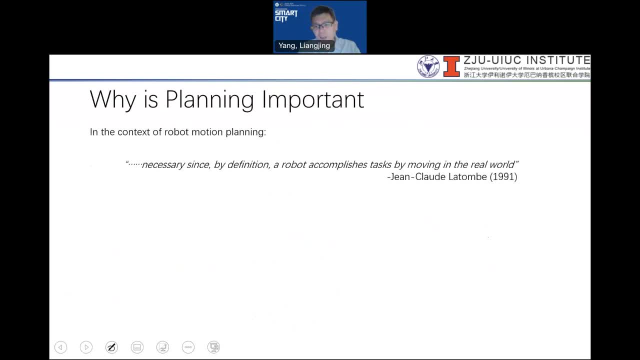 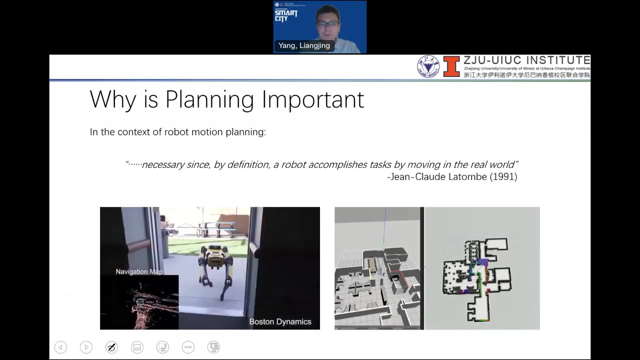 Is it necessary to plan? Yeah, A lot of other ways Okay, In the context of robotic Motion can be necessarily important. Okay, By definition, robot task by Okay. so these are some of the okay. So, uh, I would like you to think about some of this, uh.